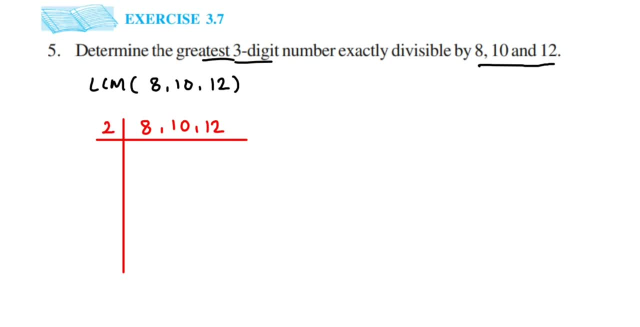 Like 2, 2 can divide all these three numbers right. So 2- 4s are 8, 2- 5s are 10 and then 2- 6s are 12.. Again, I will take a 2 because it can divide 4 and 6.. So 2- 2s are 4, 5 we. 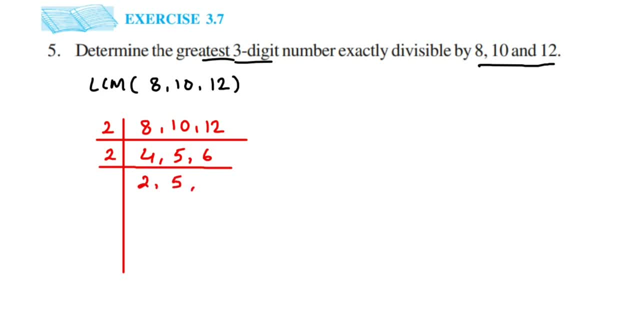 cannot divide, so write it like that. and then 2, 3s are 6.. Now we got all the three prime numbers, which doesn't go in any other table except itself. So 2 ones are 2, and then 5 and then 3.. Again, I will take 3 now. So 1 will get 5 and 3 ones. 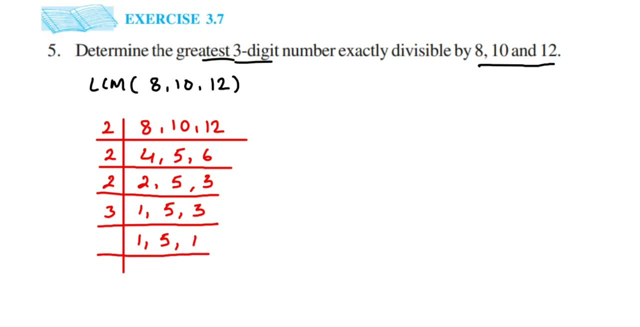 are 3.. Again we have 5. so 5 ones are 5.. That's it. So once you got 1 at the end, stop it. So LCM will be multiply all these factors, So LCM will be equal to 12.. So once you have, 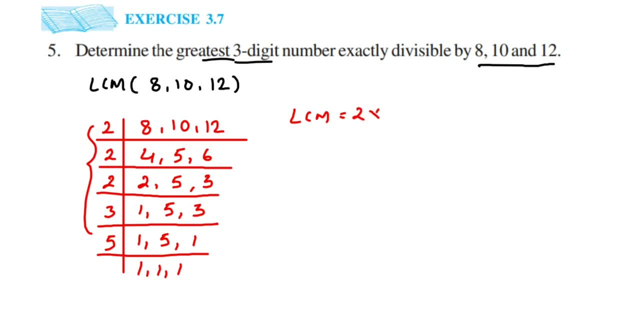 two into two, into two, into three, into five. now it's like two, twos are four, four, twos are eight. eight is a twenty four. twenty four, five is a one twenty. so lcm is one twenty. but if you observe here one twenty is a smallest three digit number, like it's a least common multiple here in the 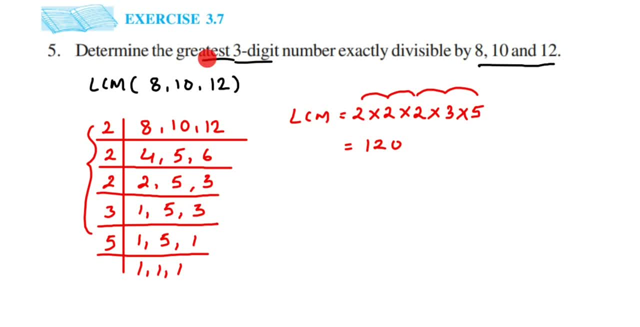 question. we want the greatest three digit number. so what we're going to do here we're going to check the table of 120 and from there we're gonna see which was the greatest three digit number. okay, we have to check the 120 table. now, instead of checking 120 table, I will check the 12 table. 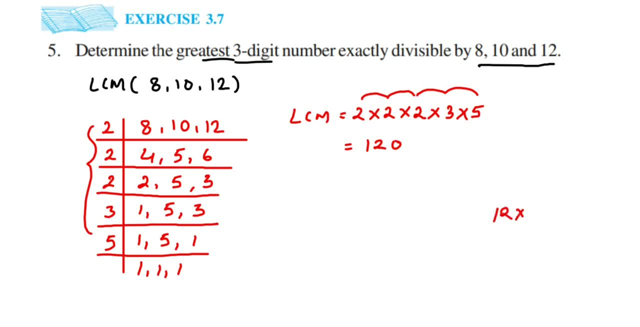 we know that 12 nines are is 108, which means 120 nines are will be 109, 080. it is a four digit number. no, we want three digit number. and we also know that 12 eights are is 96. then 128, sir, will be 960. so after 960, next number is 1080. so the small, the greatest, three.